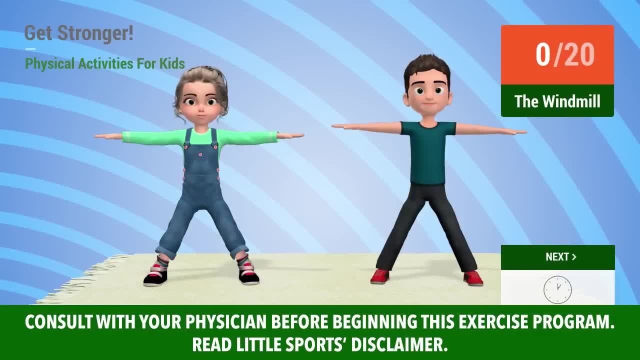 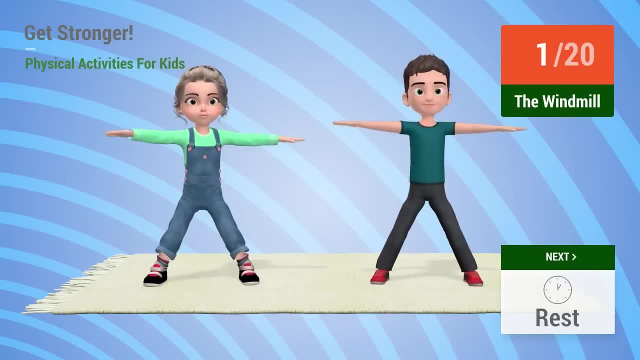 Up next the windmill In 5,, 4,, 3,, 2, 1, go 1,, 2,, 3,, 4,, 5,, 6,, 7,, 8,, 9, 10. 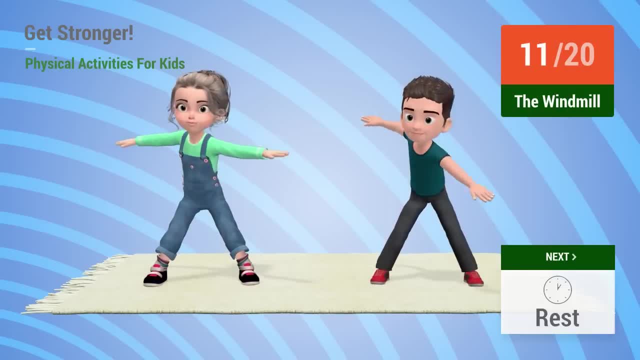 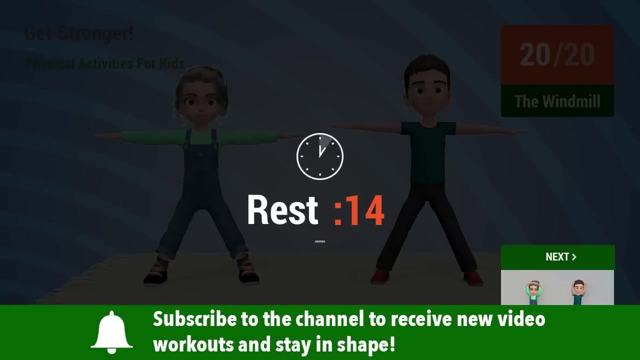 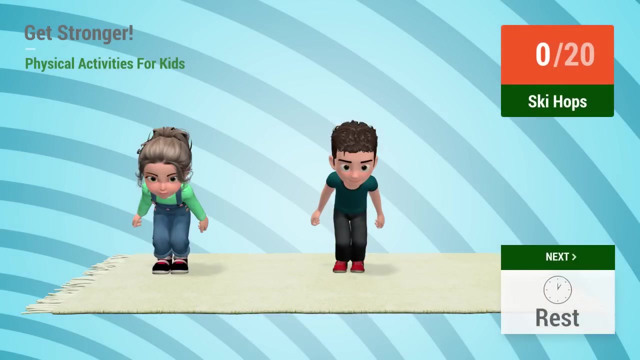 11,, 12,, 13,, 14,, 15,, 16,, 17,, 18,, 19, 20 Rest time. Up next ski hops In 5,, 4,, 3,, 2,, 1, go. 1,, 2,, 3,, 4,, 5,, 6,, 7,, 8,, 9,, 10, 11,, 12,, 13,, 14,, 15,, 16,, 17,, 18,, 19, 20. 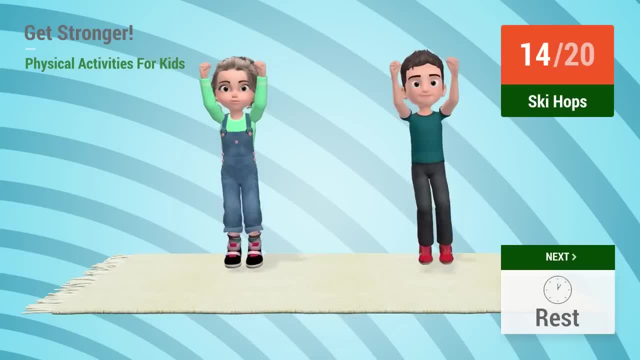 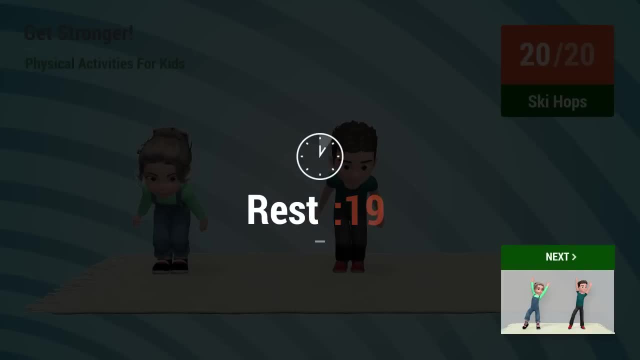 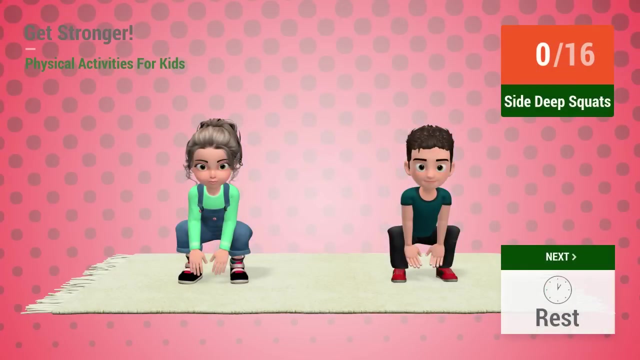 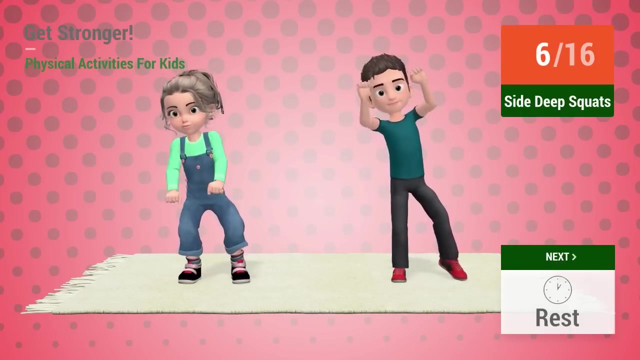 Rest time. Up next side deep squats In 5,, 4,, 3,, 2,, 1, go 1,, 2,, 3,, 4,, 5,, 6,, 7,, 8,, 9, 10. 11,, 2,, 3,, 4,, 5,, 6,, 7,, 8,, 9, 10, 11,, 2,, 3,, 3,, 3,, 4,, 5,, 6,, 7,, 8,, 9, 10. 4,, 3,, 4,, 5,, 6,, 7, 10, 15, 16, time. 1,, 2,, 3,, 4,, 5,, 6,, 7,, 9, 10. 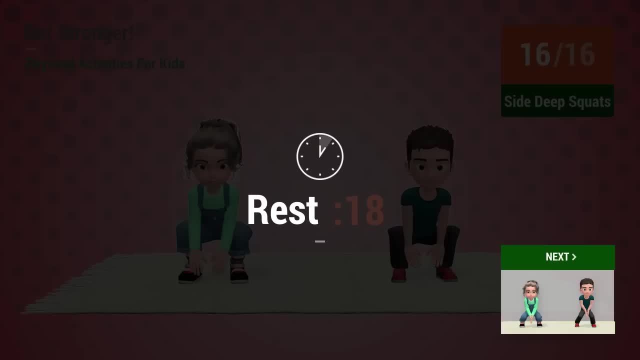 Rest time. Stay in position for 15 seconds, if needed, In 6,, 4,, 5,, 6,, 7,, 8,, 9,, 10,, 10,, 11,, 12,, 13,, 14,, 15,, 16,, 17,, 18,, 20,, 21,, 22,, 23,, 24,. 22,, 23,, 24,, 25,, 26,, 27,, 28,, 29,, 30 days. Stay in position for 15 to 22 hours each week. Stay in position for 54 hours each week. 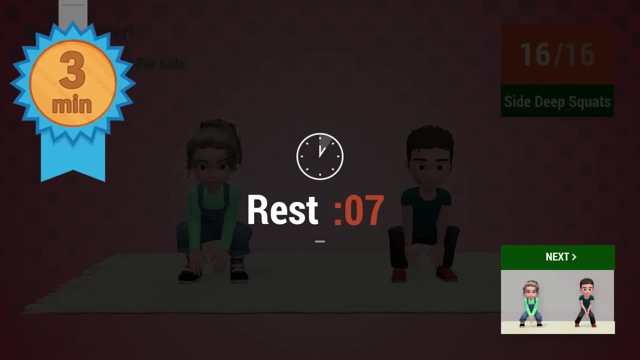 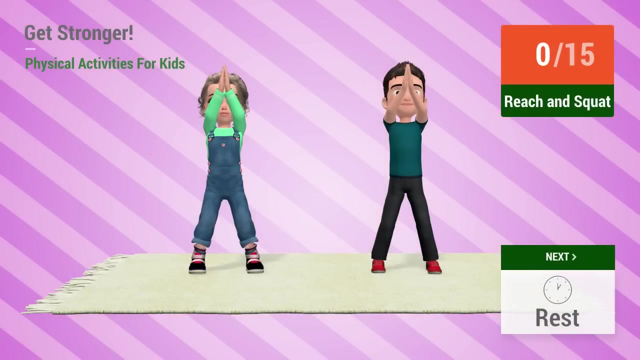 Next leg: Stay in position for 39 hours each week. You're three minutes in Good job and keep exercising Up. next, reach and squat in 5,, 4,, 3, 2, 1.. Go 2, 1, 2, 3, 4, 5, 6, 7,, 8,, 9,, 10,, 11,, 12,, 13,, 14, 15.. 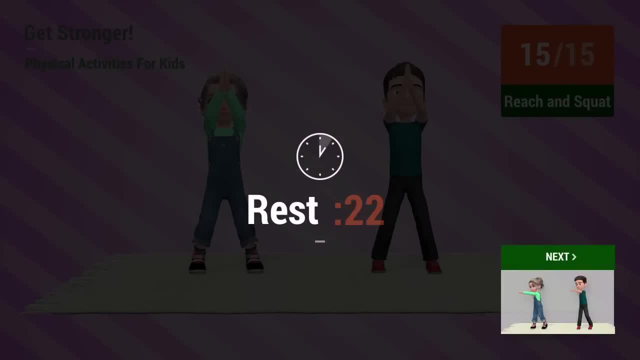 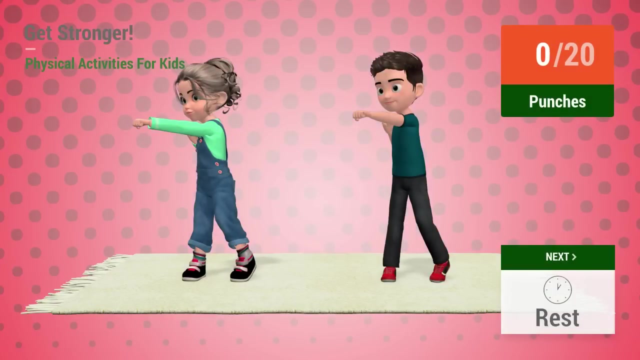 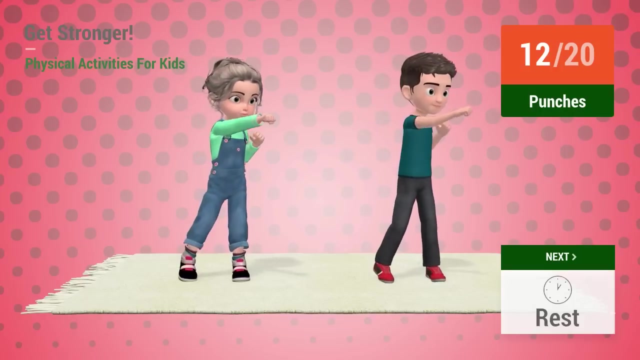 Rest time. Up next. punches in 5,, 4,, 3,, 2, 1.. Go Up next. punches in 5,, 4,, 3,, 2, 1.. Go 1,, 2,, 3,, 4,, 5,, 6,, 7,, 8,, 9,, 10,, 11,, 12,, 13,, 14,, 15,, 16,, 17,, 18,, 19, 20.. 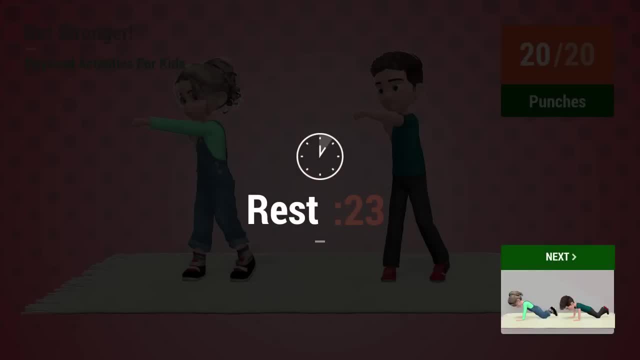 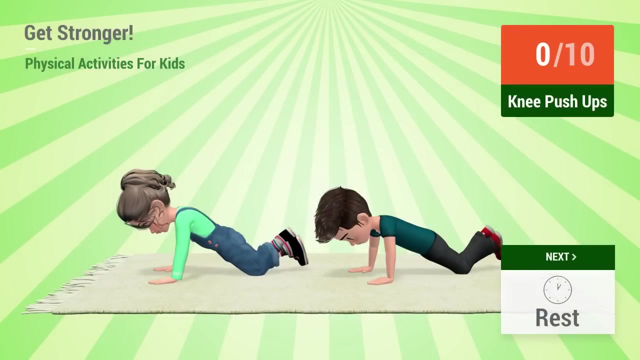 Rest time. Up next knee push-ups In 5,, 4,, 3,, 2, 1.. Go 1, 2, 3, 4,, 5,, 6,, 7,, 8,, 9,, 10,, 11,, 12,, 13,, 14, 15.. 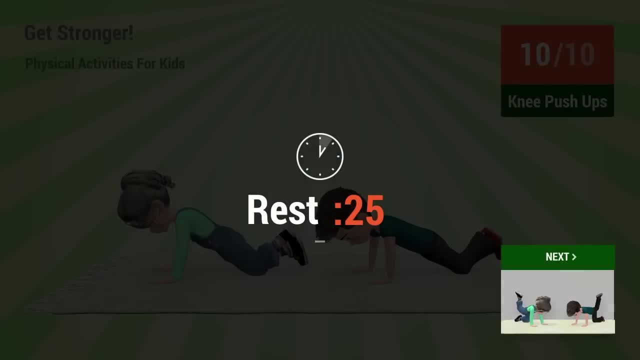 Rest time. Up next, push and squat in 5,, 4,, 3,, 2,, 1.. Go 2, 1,, 2,, 3,, 4,, 5,, 6,, 7,, 8,, 9,, 10,, 11,, 12,, 13,, 14,, 15.. 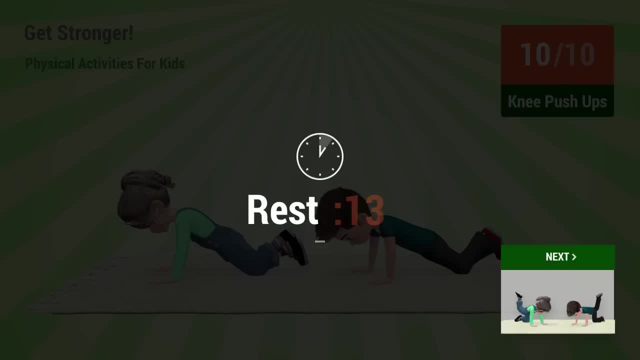 Rest time In 5,, 4,, 3,, 2, 1.. Go 1,, 2,, 3,, 4,, 5,, 6,, 7,, 8,, 9,, 10,, 11,, 12,, 13,, 14,, 15.. 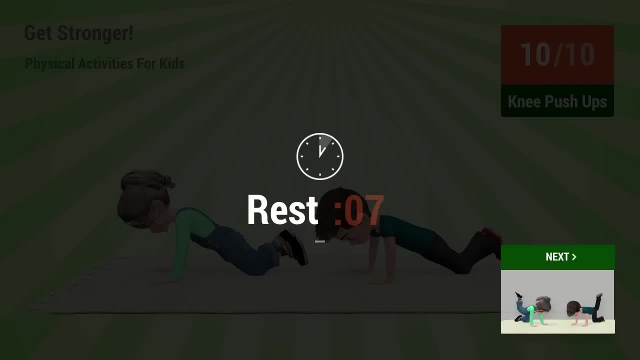 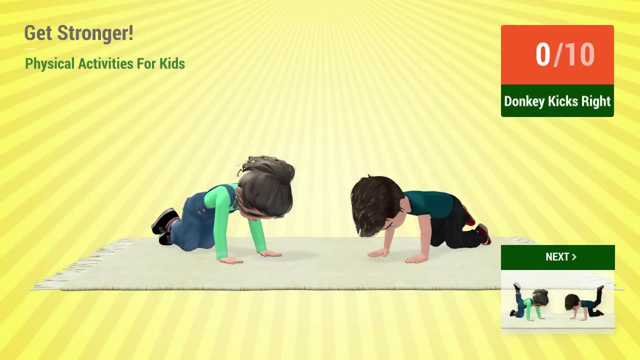 Rest time In 5,, 4,, 3,, 2, 1.. Go In 5,, 4,, 2, 1. Go Rest time. Rest time Up next donkey kicks in 5,, 4,, 3,, 2,, 1, go. 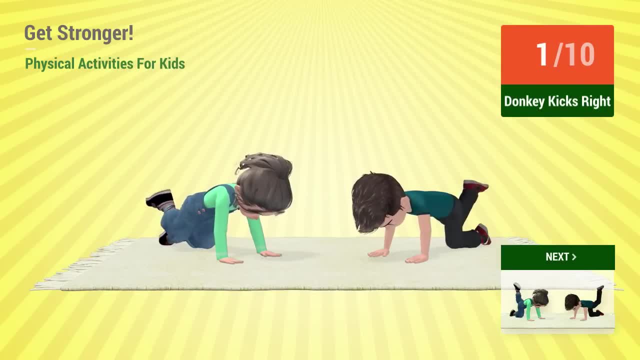 1,, 2,, 3,, 4,, 5,, 6,, 7,, 8,, 9,, 10, up. next, donkey kicks in 5,, 4,, 3,, 2,, 1, go. 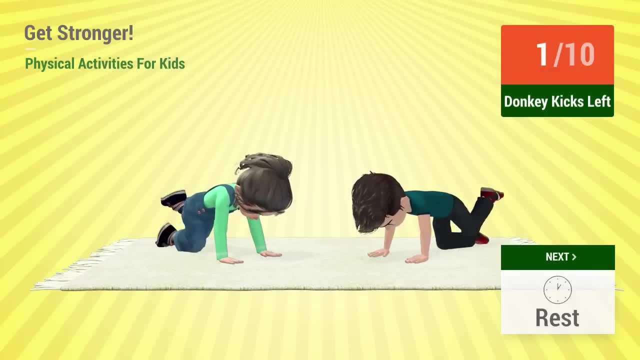 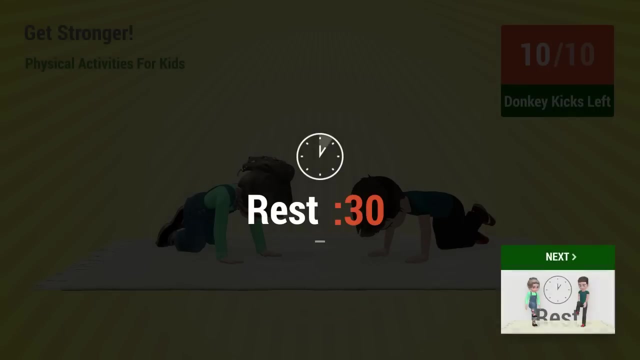 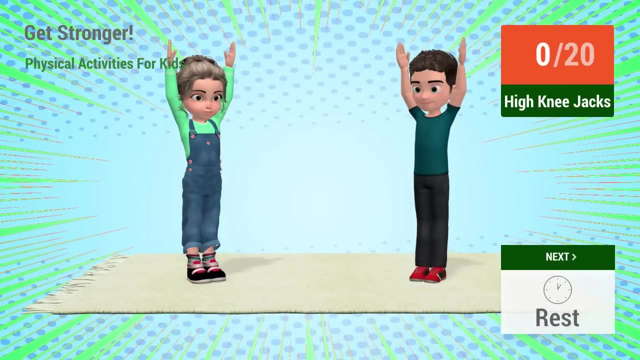 1,, 2,, 3,, 4,, 5,, 6,, 7,, 8,, 9,, 10, rest time. Up next high knee jacks in 5,, 4,, 3,, 2,, 1, go. 1,, 2,, 3,, 4,, 5,, 6,, 7,, 8,, 9,, 10,, 11,, 12,, 13,, 14,, 15,, 16,, 17,, 18,, 19,, 20,, 21,, 22,, 23,, 24,, 25,, 26,, 27,, 28,, 29,, 30,, 31,. 32,, 33,, 34,, 35,, 36,, 37,, 38,, 39,, 40,, 41,, 42,, 43,, 44,, 45,, 46,, 47,, 48,, 49,, 50,, 51,, 52,, 53,. 54,, 55,, 56,, 57,, 58,, 59,, 52,, 53,, 54,, 55,, 56,, 57,, 58,, 59,, 52,, 53,, 54,, 56,, 57,, 58,, 59,, 52,, 53,. 56,, 58,, 59,, 52,, 53,, 54,, 55,, 56,, 57,, 58,, 59,, 52,, 53,, 53,, 54,, 55,, 56,, 57,, 58,, 59,, 52,, 53,. 56,, 58,, 59,, 52,, 53,, 53,, 53,, 54,, 55,, 56,, 57,, 58,, 59,, 52,, 53,, 53,, 54,, 56,, 57,, 58,. 56,, 58,, 59,, 52,, 53,, 53,, 54,, 56,, 57,, 58,, 59,, 52,, 53,, 53,, 54,, 56,, 57,, 58,. 58,, 59,, 52,, 53,, 54,, 56,, 58,, 59,, 52,, 53,, 55,, 56,, 57,, 56,, 57,, 56,, 57,, 58,. 56,, 59,, 52,, 53,, 54,, 53,, 54,, 56,, 57,, 54,, 55,, 49,, 55,, 56,, 57,, 58,, 59,, 54,, 56,, 58,. 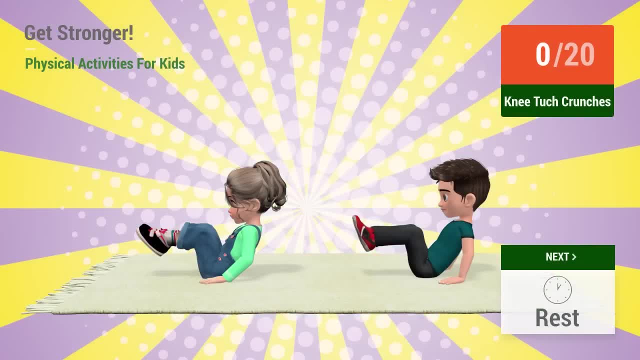 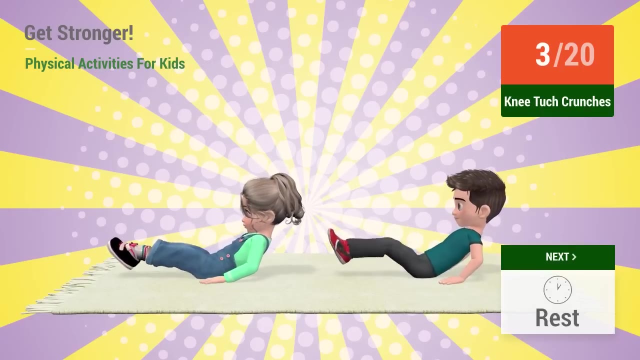 57, GOOD required. great with confidence. Up next knee tuck crunches in 5,, 4,, 3,, 2, 1.. Go 1,, 2,, 3,, 4,, 5,, 6,, 7,, 8,, 9,, 10,, 11,, 12,, 13,, 14,. 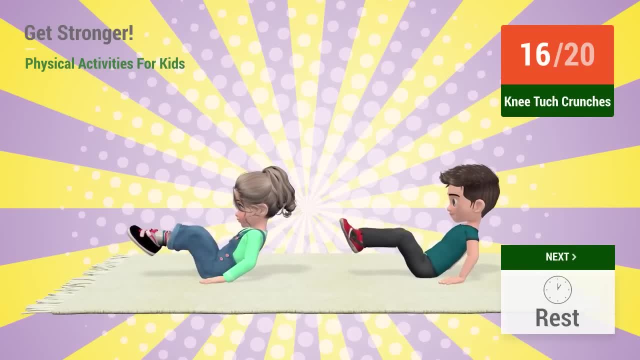 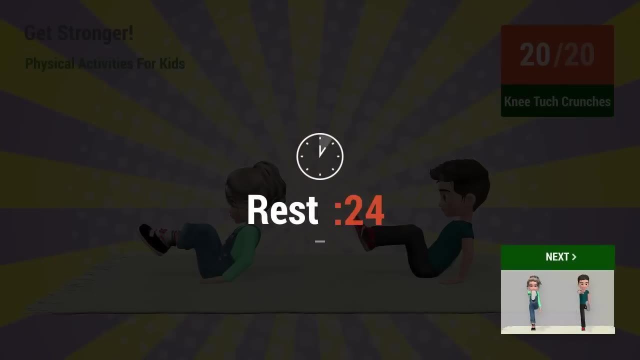 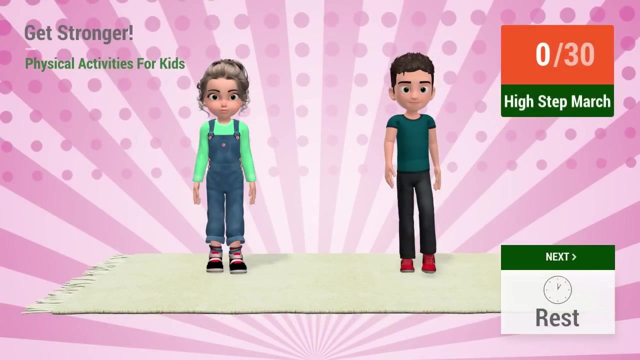 15,, 16,, 17,, 18,, 19, 20.. Rest time Up next high step march in 5,, 4,, 3,, 2, 1. Go 1,, 2,, 3,, 4,, 5,, 6,, 7,, 8,, 9,, 10,, 11,, 12,, 13,, 14,, 15,, 16,, 17,, 18,, 19,, 20.. 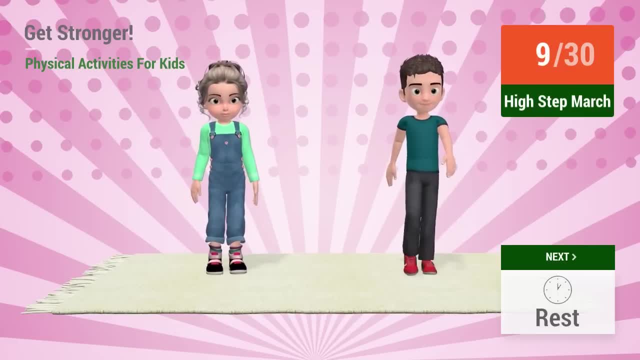 Up next knee. tuck crunches in 5,, 4,, 3,, 2,, 1.. Go 1,, 2,, 3,, 4,, 5,, 6,, 7,, 8,, 9,, 10,, 11,, 12,, 13,, 14,, 15,, 16,, 17,, 18,, 19, 20.. 21,, 22,, 23,, 24,, 25,, 26,, 27,, 28,, 29,, 30.. 21,, 22,, 23,, 24,, 25,, 26,, 27,, 28,, 29,, 30.. 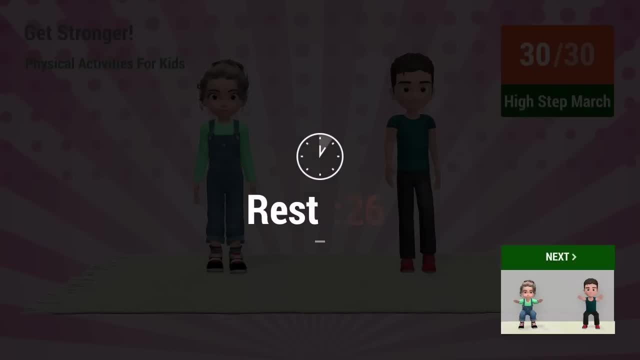 Rest time: 1,, 2,, 3,, 4,, 5,, 6,, 7,, 8,, 9,, 10,, 11,, 12,, 13,, 18,, 19, 20.. 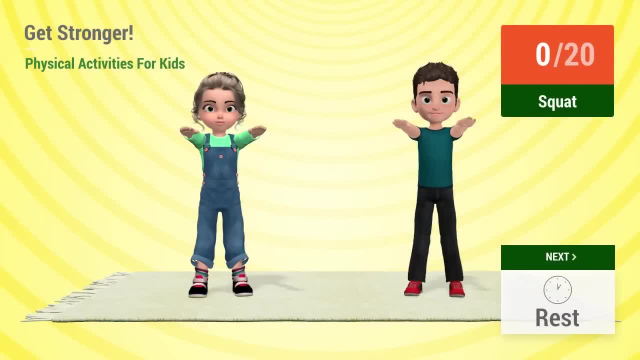 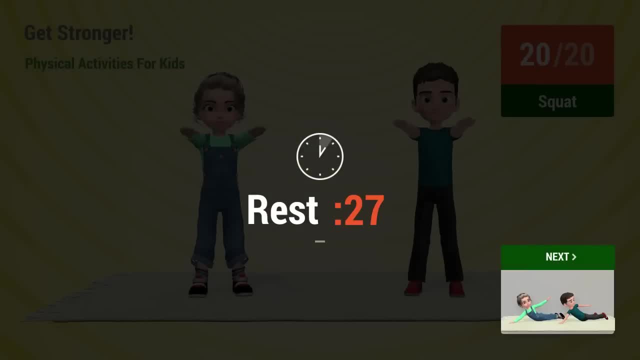 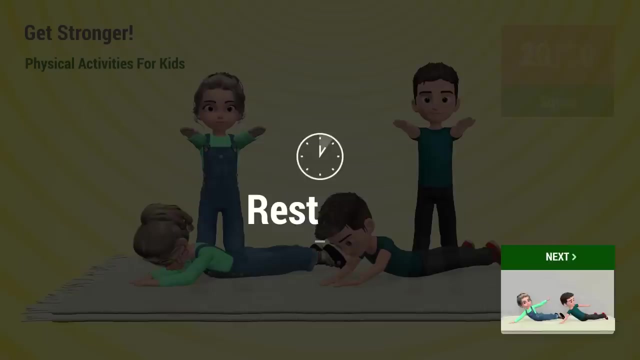 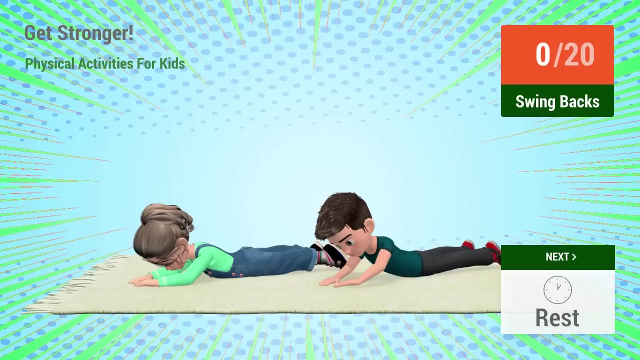 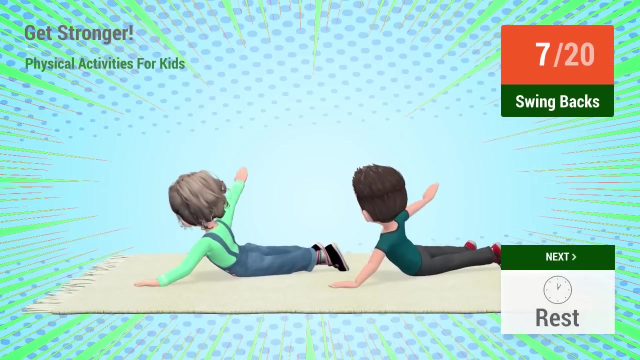 Rest time. Up next swing backs in: 5,, 4,, 3,, 2,, 1, go 1,, 2,, 3,, 4,, 5,, 6,, 7,, 8,, 9,, 10,, 11,, 12,, 13,, 14,, 15,, 16,, 17,, 18,, 19, 20.. 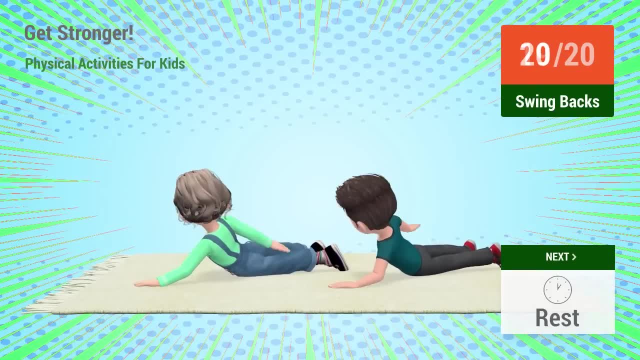 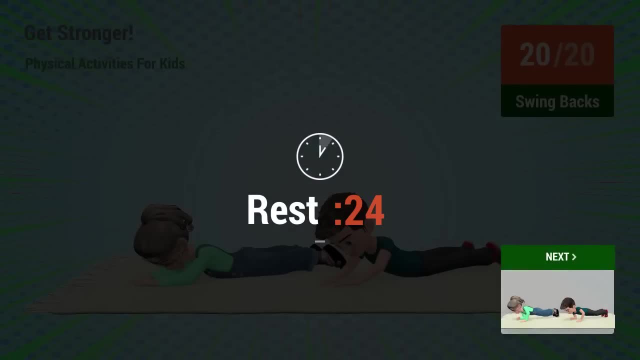 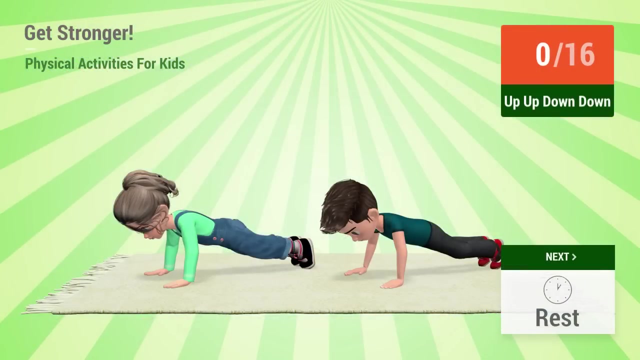 18, 19, 20, rest time Up next up, up, down down in 5,, 4,, 3,, 2, 1, go 1, 2,, 3,, 4,, 5,, 6,, 7,, 8,, 9,, 10,, 11,, 12,, 13,, 14,, 15,, 16,, 17,, 18,, 19,, 20.. 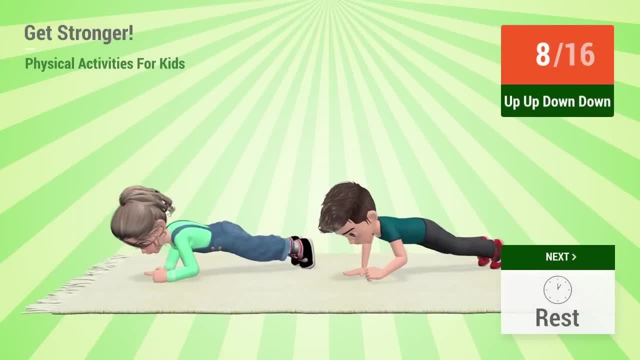 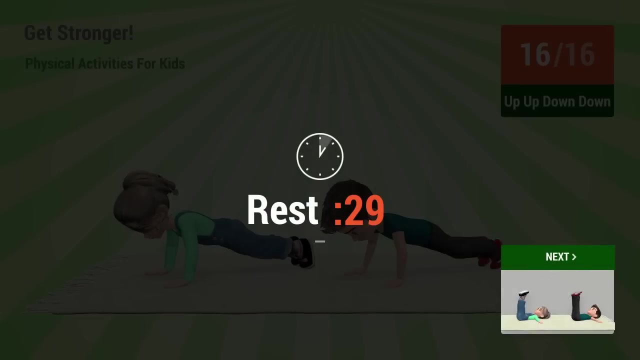 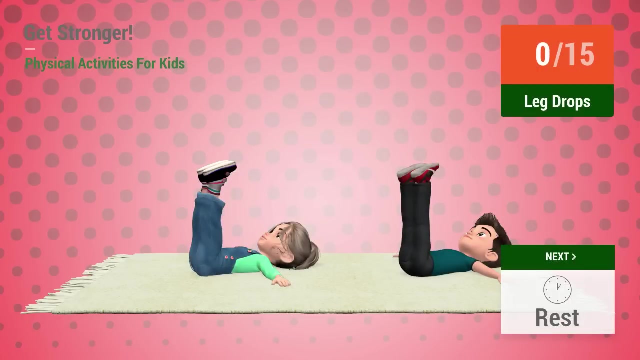 7,, 8,, 9,, 10,, 11,, 12,, 13,, 14,, 15,, 16,. rest time: 1,, 2,, 3,, 4,, 5,, 6,, 7,, 8,, 9,, 10,, 12,, 13,, 18,, 19, 20.. 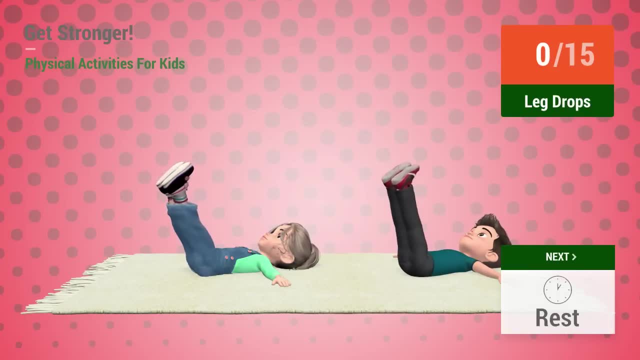 1,, 2,, 3,, 4,, 5,, 6,, 7,, 8,, 9,, 10,, 11,, 12,, 13,, 18,, 19,, 20.. 10,, 11,, 12,, 13,, 14,, 15, rest time.